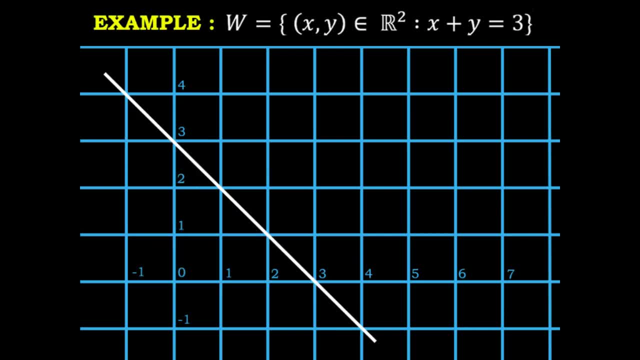 vectors that form this line. By joining all these arrowheads, we get the graph of the given set Out of all the vectors that form this line. let's randomly pick any two of the vectors. The sum of these two vectors gives us a third vector. This new vector, however, is not a part. 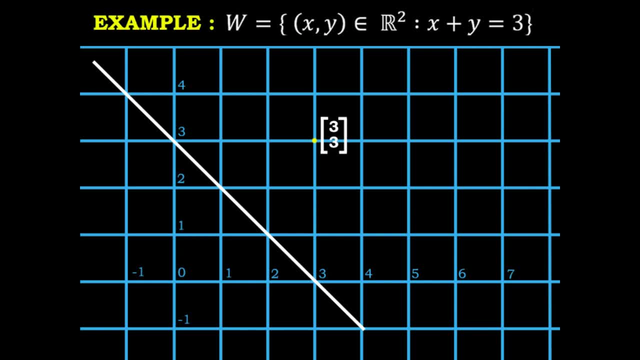 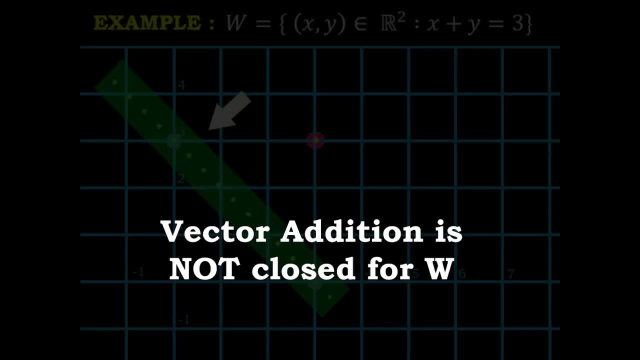 of the line that represents the given set, In other words, the sum of any two random vectors in the set may not be a part of the given set of vectors. So vector addition for the given set is not closed, and so the given set does not form a vector space. 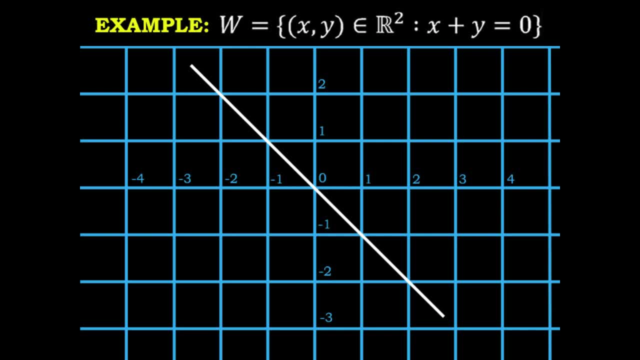 This is what the graphical representation of the given set looks like. Every point on this line is a vector. If we replace all these points by pointed arrows with their tails at the origin and their heads at the points on the given line, then we end up getting a graphical representation of the vectors that form this line. 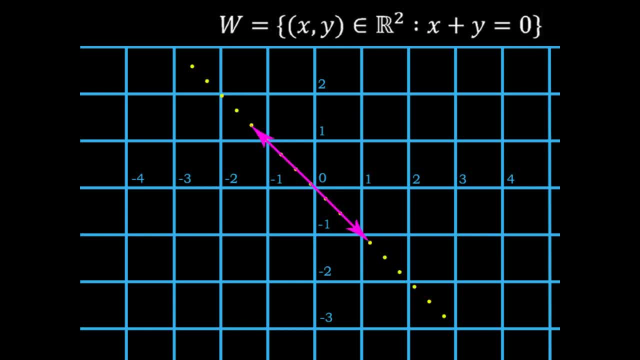 Adding any two of these vectors or multiplying any vector by a scalar gives us another vector from the same collection of vectors. The origin through which the graph passes serves as the zero vector of the given set For any random vector with a certain magnitude and pointed towards a particular. 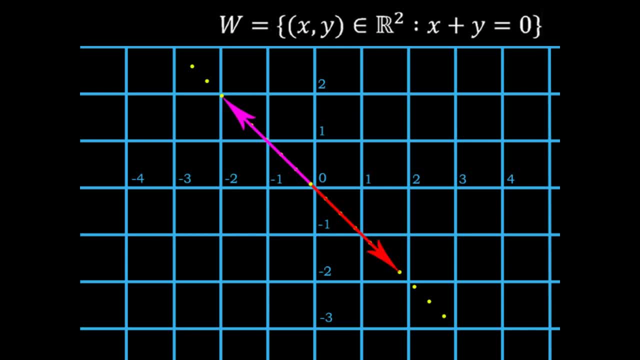 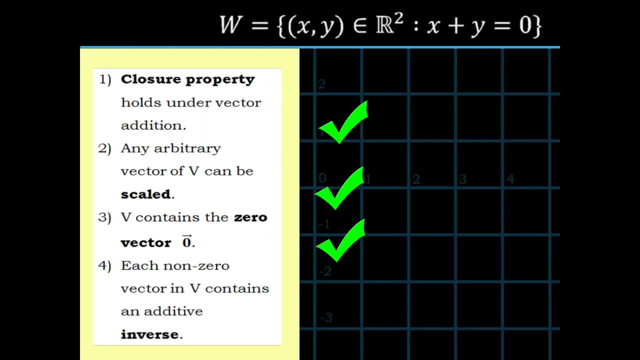 direction. there exists another vector, called the inverse of the given vector, with equal magnitude, pointed towards the exact opposite direction. Adding any vector to its inverse brings us back to the origin. So the principal conditions that form the skeleton of a vector space are satisfied by the given set. The other conditions can also be proven similarly. 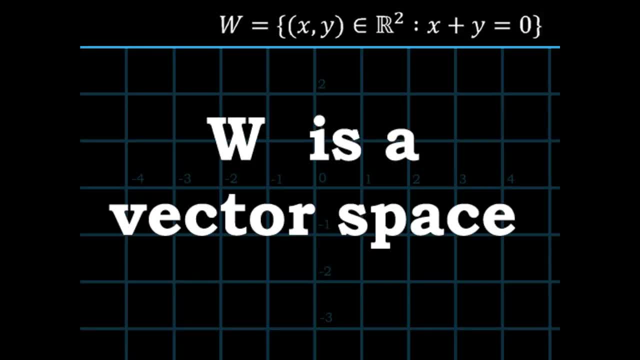 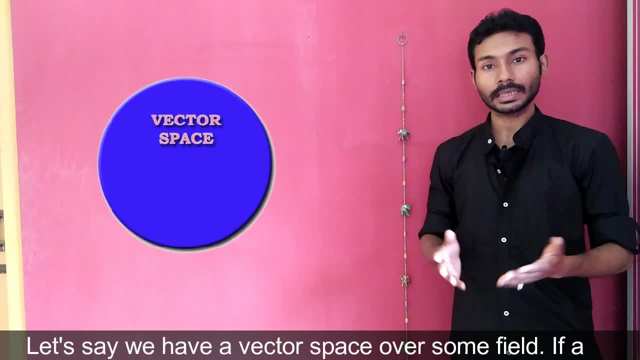 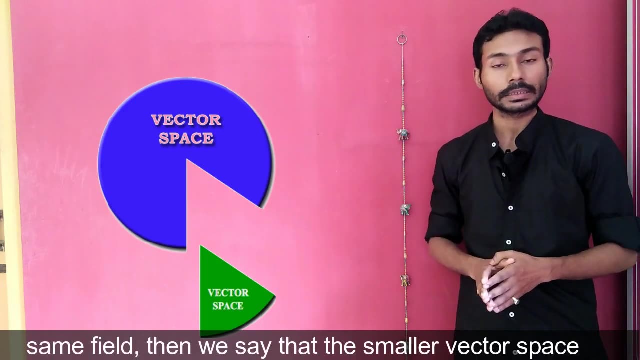 So the given set does form a vector space. Let's say we have a vector space over some field. If a part of this vector space is also a vector space over the same field, then we say that this smaller vector space is a subspace of the bigger vector space, that it's a 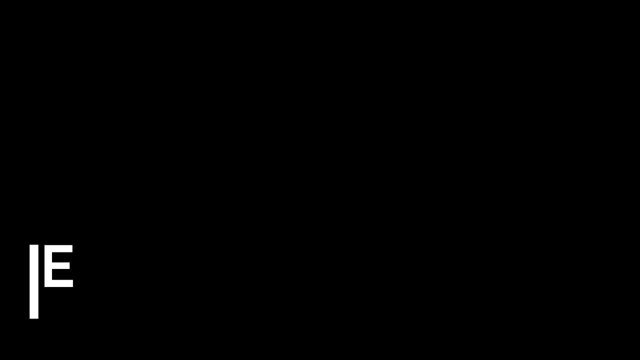 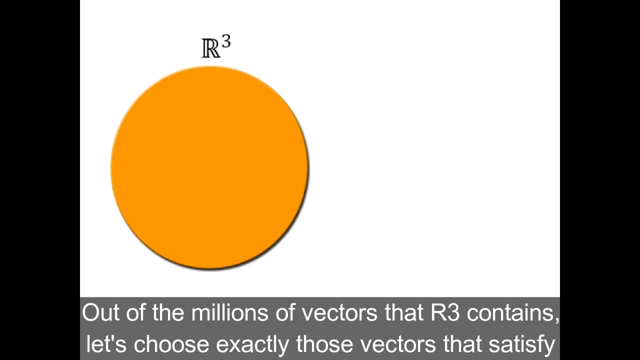 part of. Out of the millions of vectors there are three contains: let's choose exactly those vectors which satisfy, say, this condition. Let's pack the collection of all these vectors into the given set. So we need two sets into a set, say W.